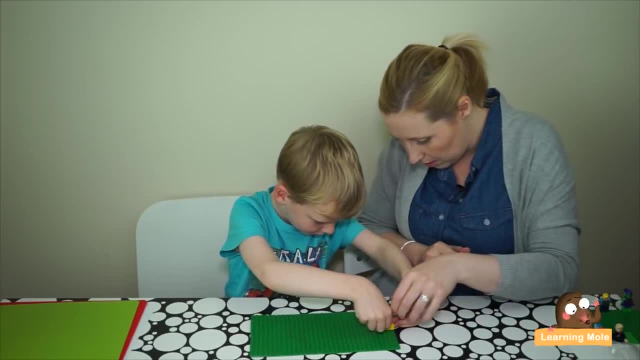 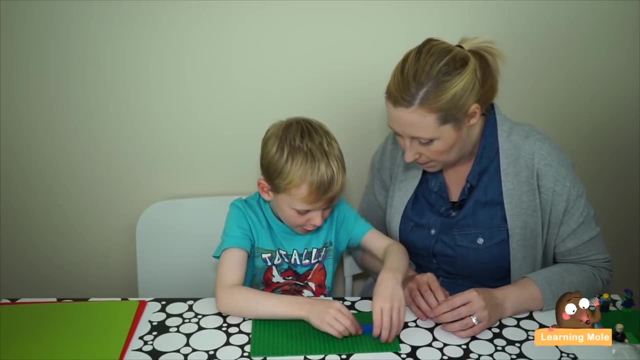 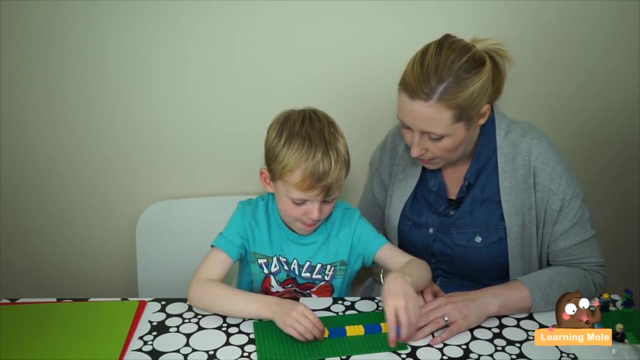 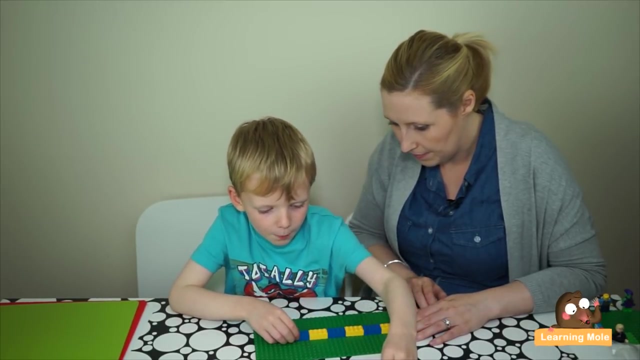 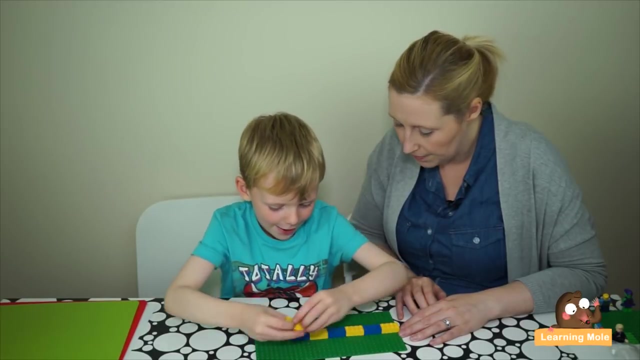 blue Yellow blue. Can you get it stuck on there? Okay, It's stuck on Yellow blue. Okay, I need another yellow Yellow blue. What's another? yellow Yellow blue, Yellow blue. I need another for yellow Yellow blue. Lovely, As you can see, you can go on all. 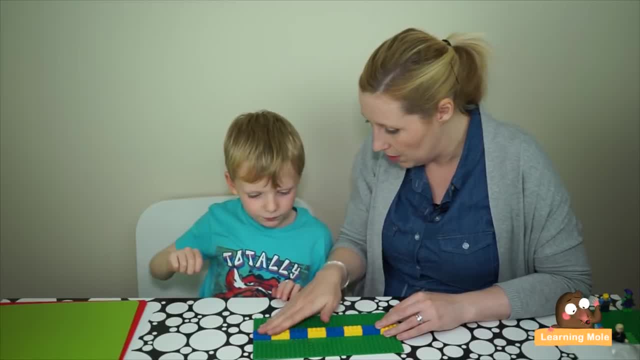 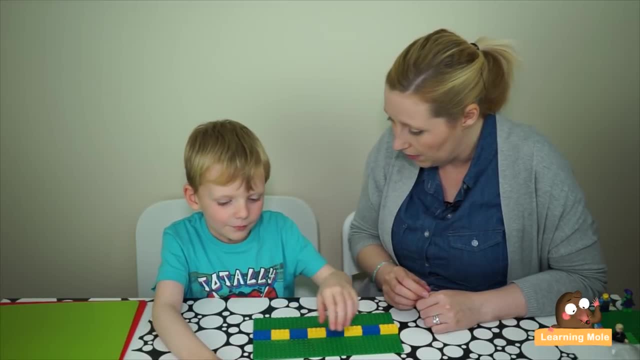 day. You can go on all day with this pattern. Okay, so that's your first pattern. This time do you think you can make a pattern with three colours? It has to have a pattern. What does a pattern have? to have The same shape. 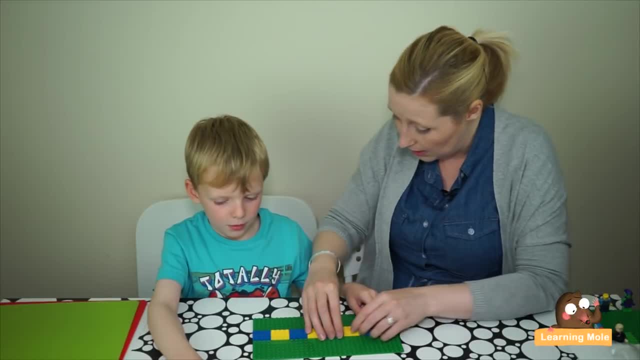 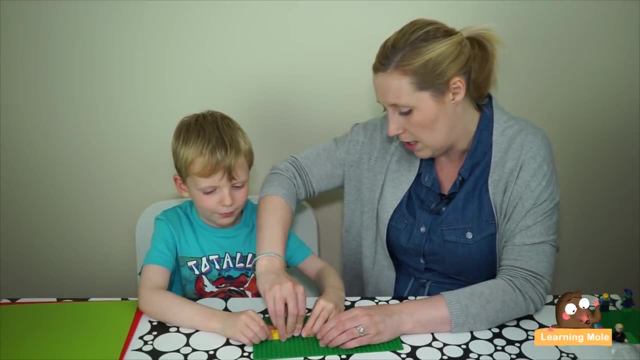 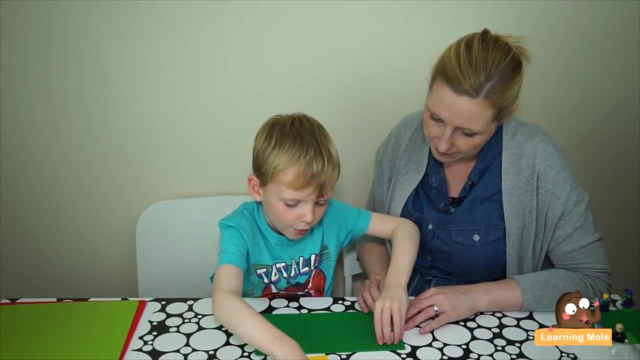 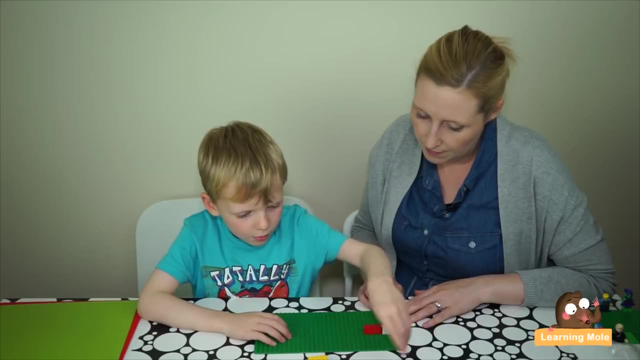 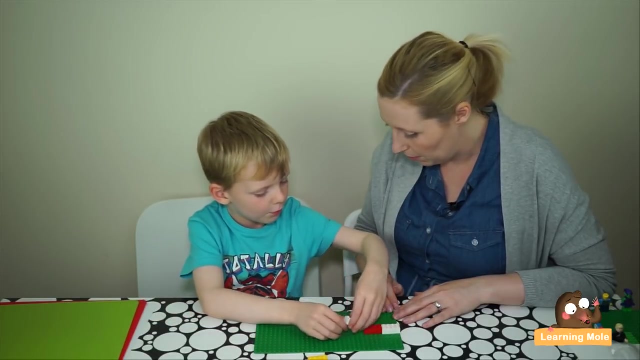 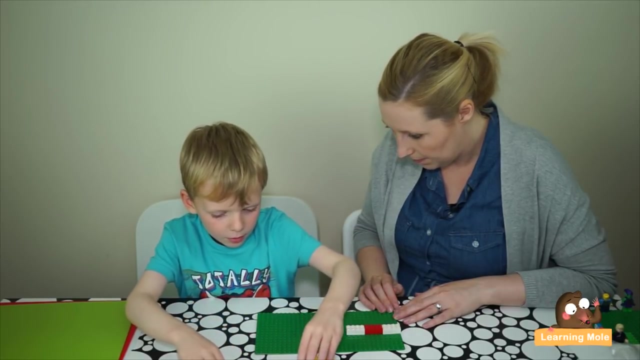 is going to be white, white, red, white. Okay, so we're going to use three colours. Yeah, white, red, white. Okay, White red, white, white, white red, white, white, red, red. 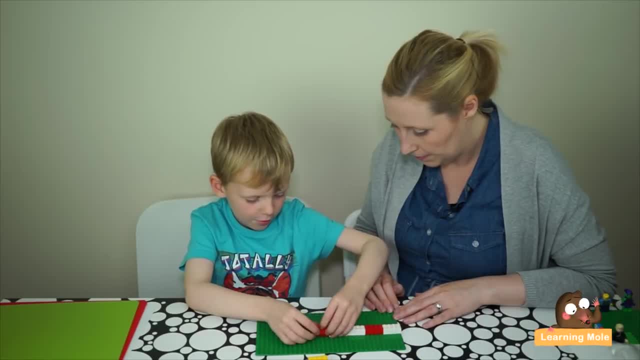 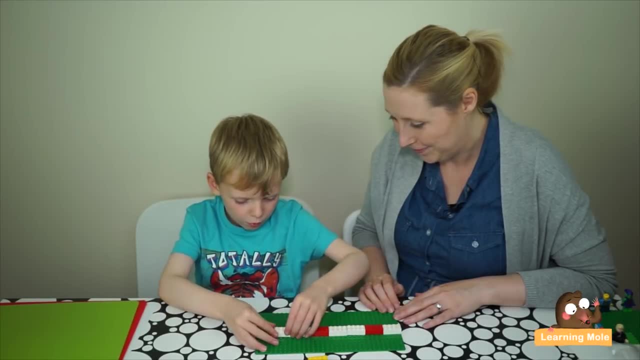 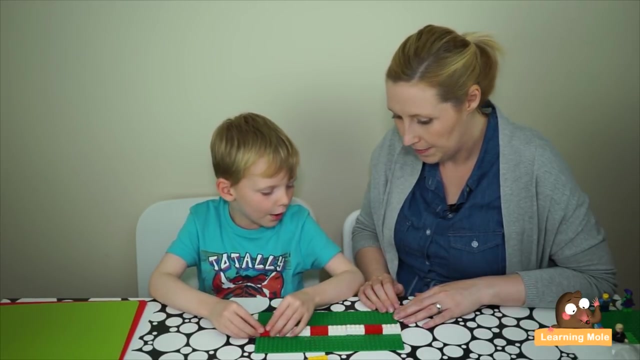 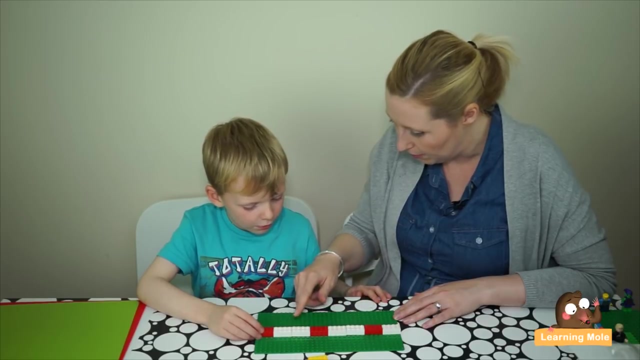 white, red, white, white, white, red. I don't have enough space to do that. Oh, so you're just putting that one in. Okay, so yours just went: white, red, white, white, red, white. 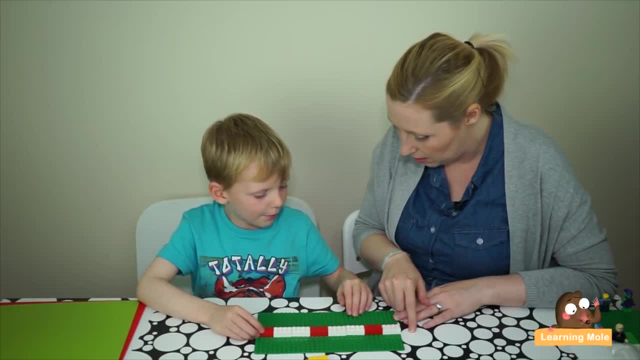 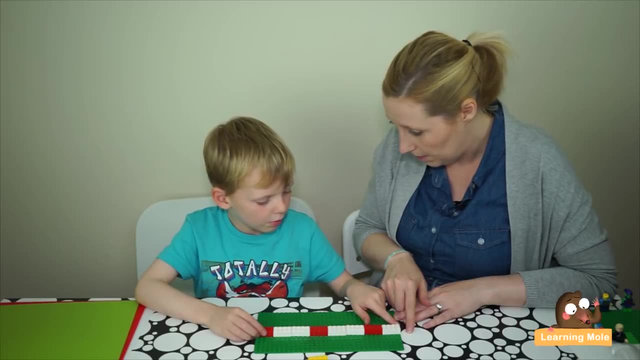 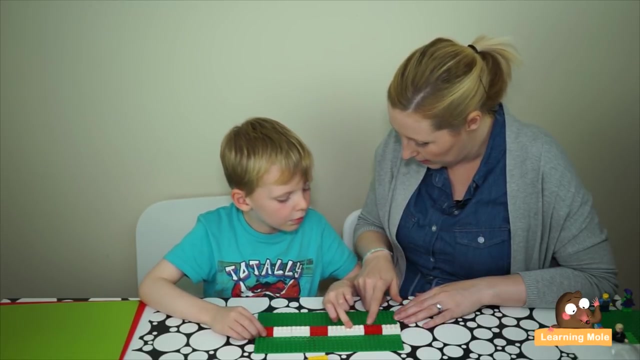 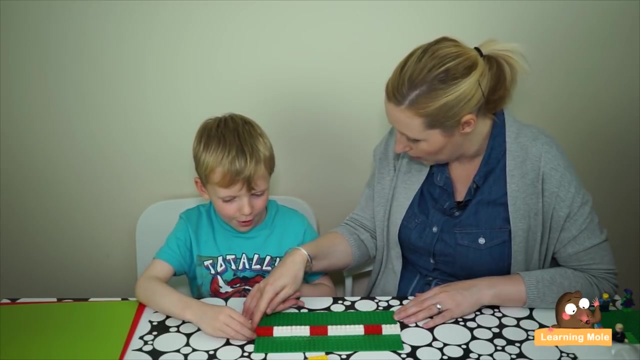 white, red. What should be here? If you could fit it on, what should be here? Red, Should it Have a think about your pattern, White, So it should be white, white Red, White, white Red, White, white, red. What? 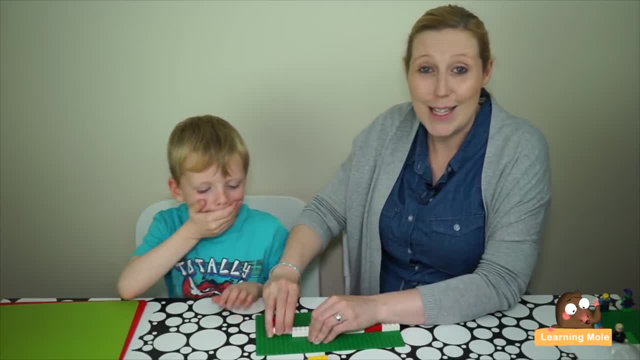 comes next? White, red, Good, okay, So again, letting them to explore what comes before and what comes after. Patterns are quite important because, although this seems very simple, you can do it any way you want. You can do it in any way you want. you can do it in any. 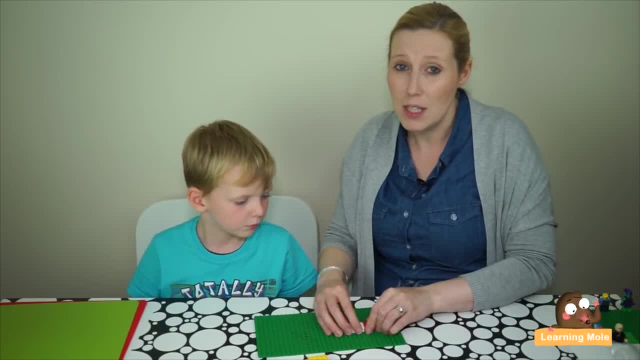 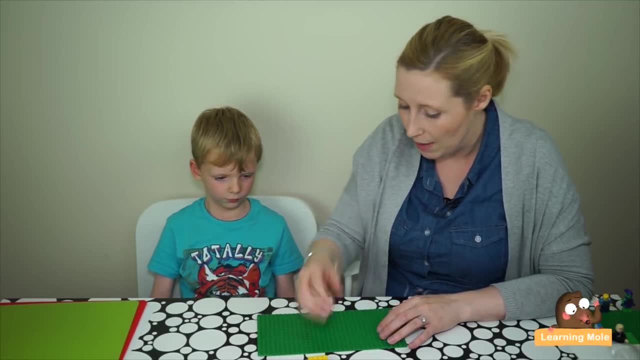 way you want. So, for example- and it's just color patterns- it actually really helps them to see patterns in numbers and relationships in numbers as they go along. So it is important to start with some pattern work early on. Okay, I'm going to give you the start of a. 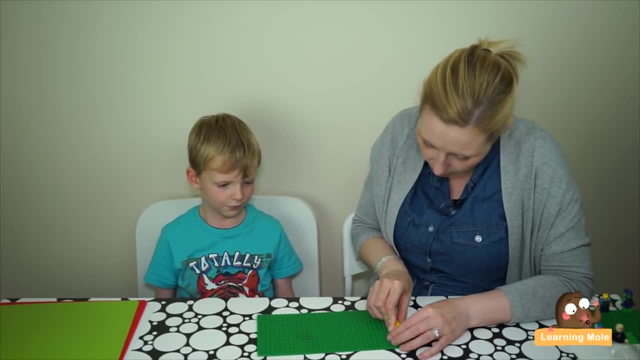 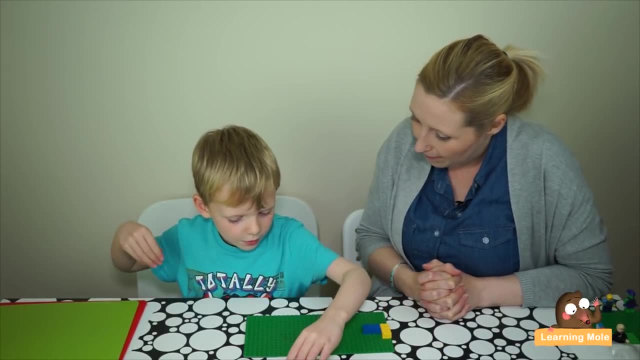 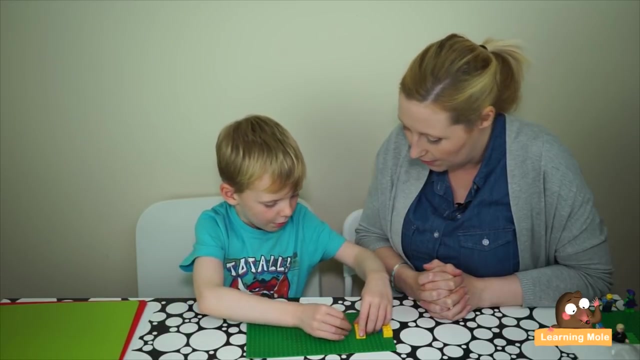 pattern this time. Now I want you to copy it and to fix the continued. Okay, This one's going to be yellow, blue. Hmm, Why are you putting it that way? Yeah, good, It's a different shape this time, isn't it A different way around? 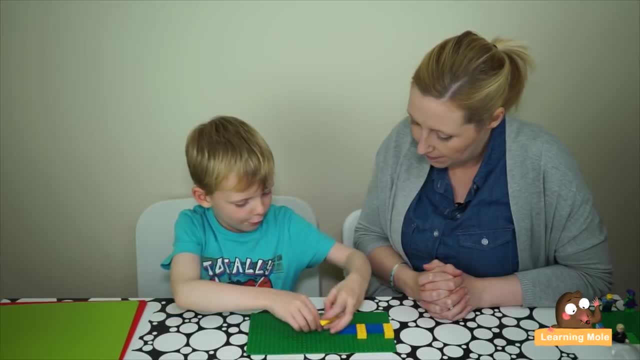 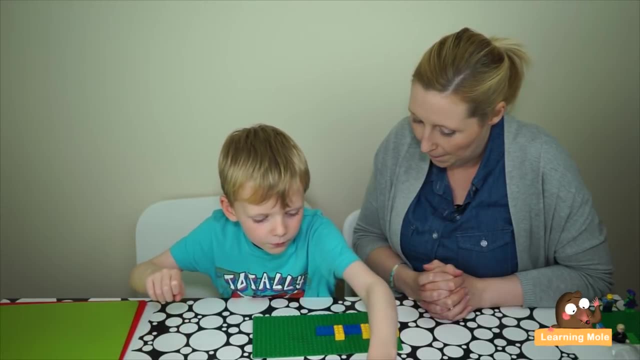 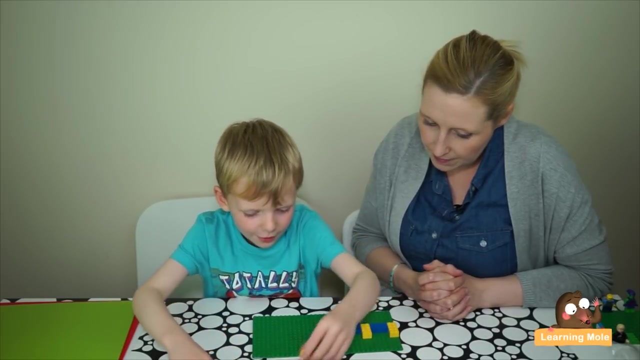 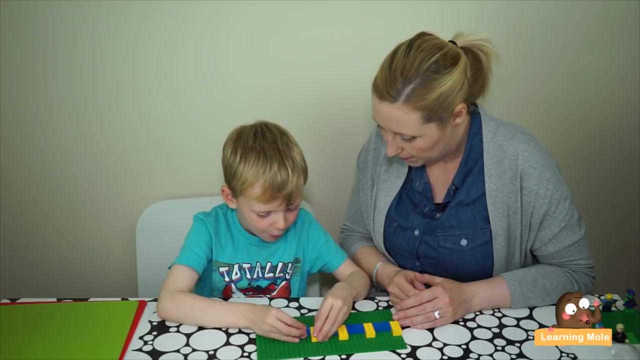 behind Yellow blue. I don't know where the yellow is Yellow. Can I do a smile? What about this one? Blue, Yellow, blue. Okay, that's enough, Good boy. well done. So again, using those shapes and making it. 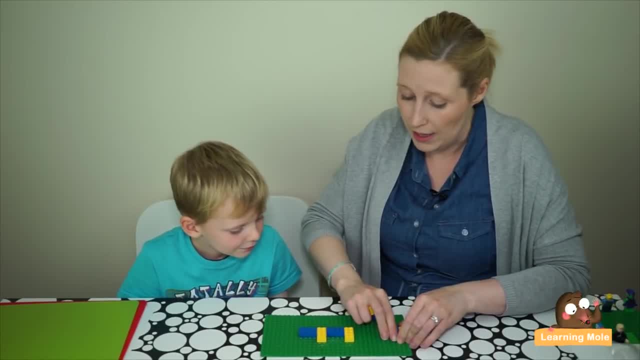 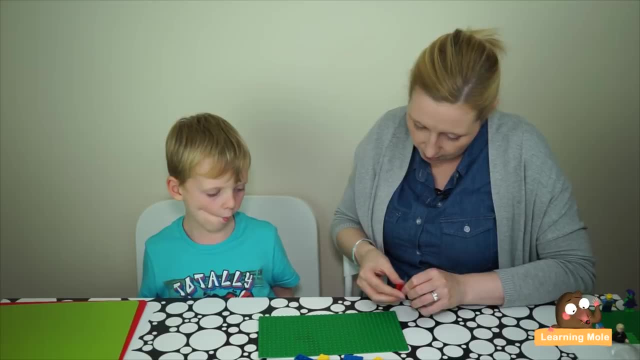 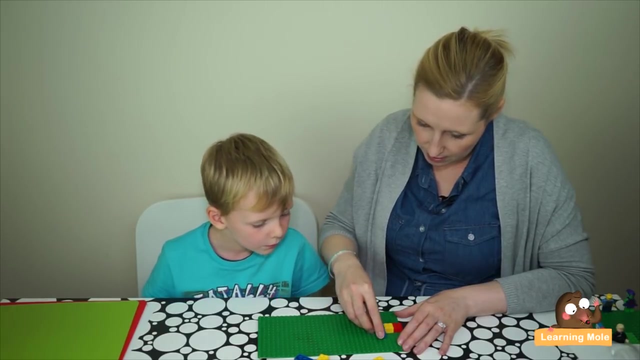 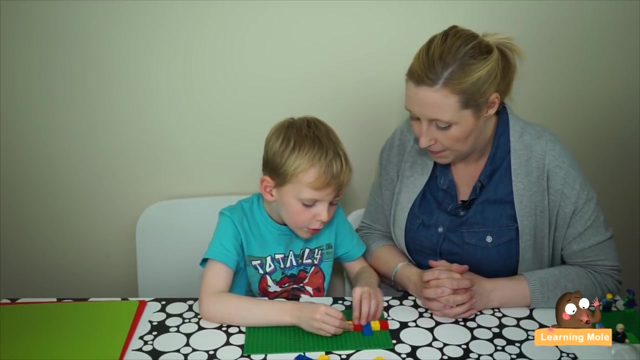 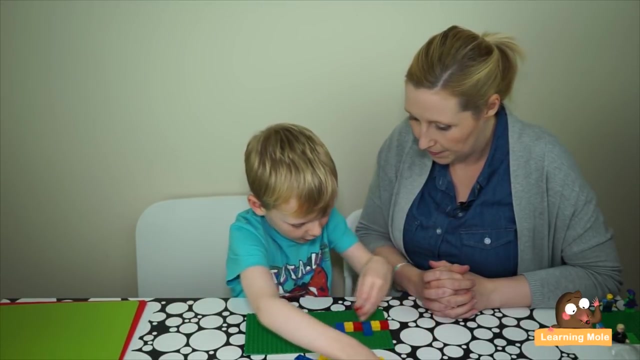 different shapes as well. so you're adding in that extra little element. Okay, you ready for the next one? Okay, this time. Okay, it's going to be red, yellow, blue, Red, Red, Yellow, blue, Red, yellow, Red, yellow, blue, blue. 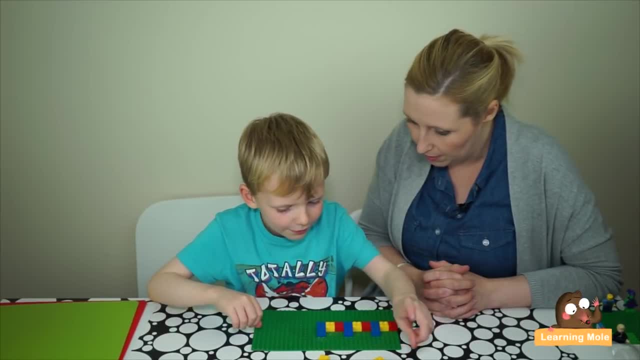 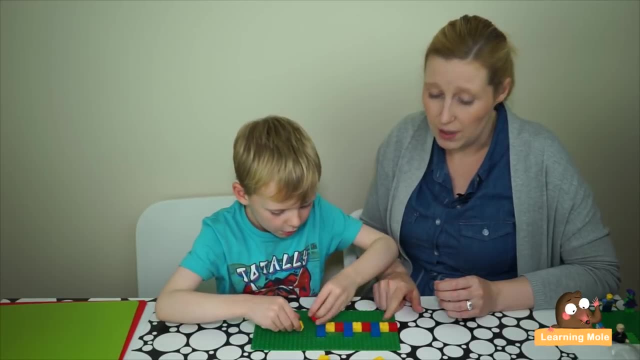 Excellent. Look carefully for another red, won't you? Can you see one? And talk about the size as well? so we've got the different sizes here, the different blocks. so it's not just about colour, it's about size, it's about the size of the. 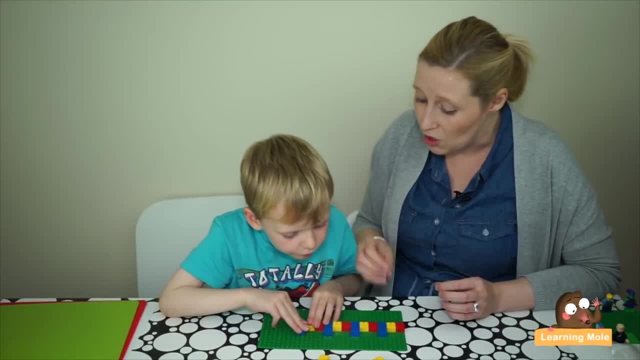 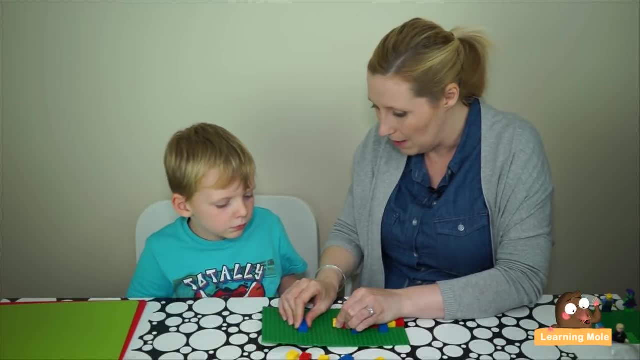 block. it's about the direction that the block is facing, it's about the shape, and it's also about the colour as well. Perfect Diane, Right. this time I'm going to build one and you're going to have to fill in the missing bits. Do you think you could do that?